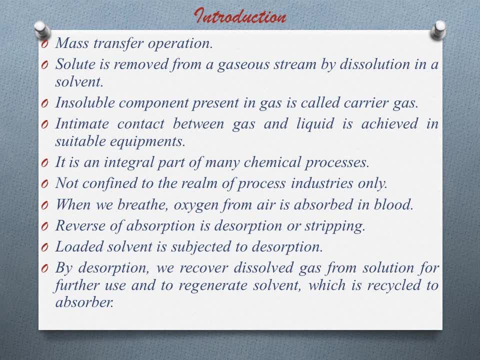 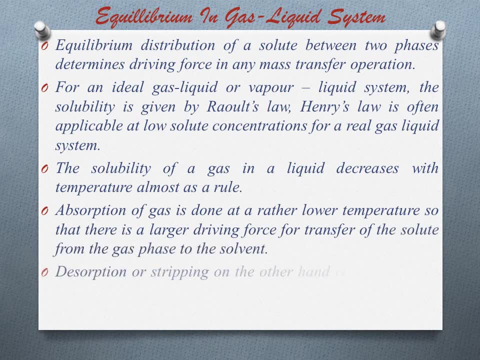 the solvent. The regenerated solvent is recycled to the absorber. Now we will discuss about the equilibrium in a gas-liquid system. A knowledge of the equilibrium distribution of a solute between two phases, ie the solubility of a species in a solvent, is very important in determining the driving force in any mass. 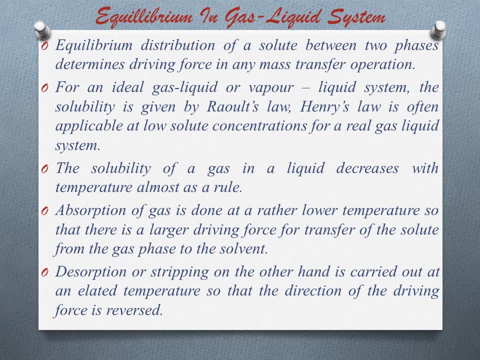 transfer operation. For an ideal gas-liquid or vapor-liquid system, the solubility is given by a Routh's law. Henle's law is often applicable at low-solute concentrations for a real gas-liquid system. The solubility of a gas in a liquid decreases with temperature. 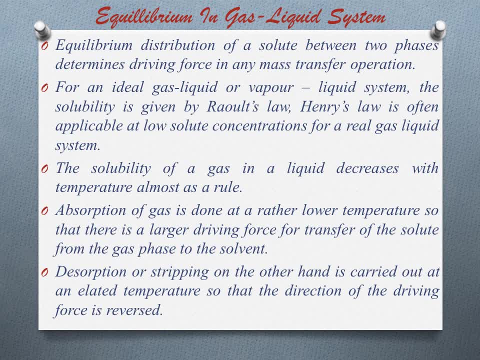 Almost as a rule, Absorption of gas is done at a rather lower temperature, so that there is a larger driving force for transfer of the solute from the gas phase to the solvent. Desorption or stripping, on the other hand, is carried out at an alienated temperature. 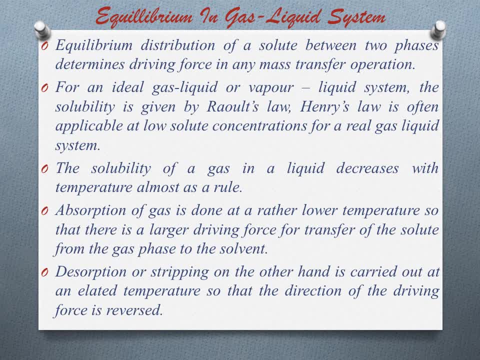 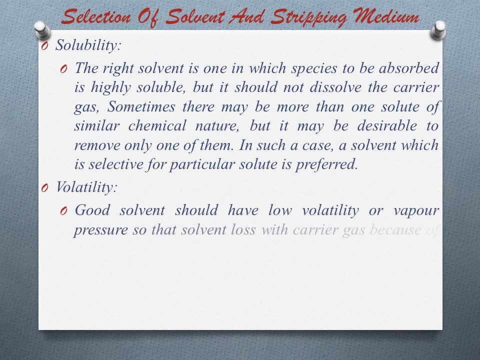 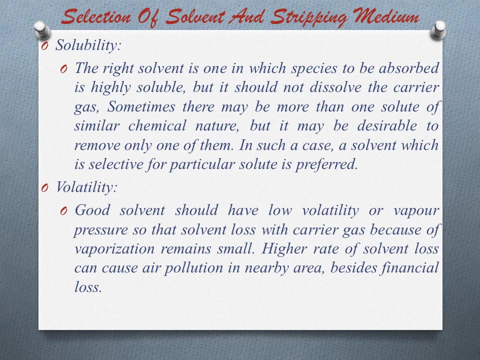 so that the direction of the driving force is reversed. Thank you, Bye, Bye. general criteria and considerations for selection of a solvent for absorption. First is solubility. The right solvent is one in which the species to be absorbed, ie the solute, is highly soluble, but it should not dissolve the carrier gas. Sometimes there 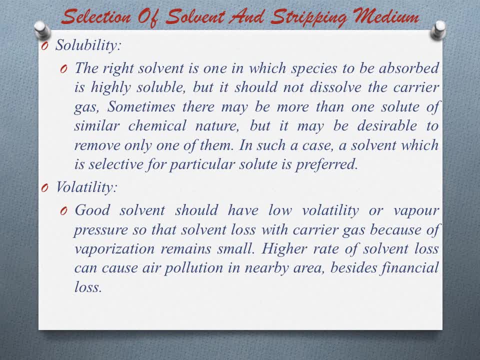 may be more than one solute of similar chemical nature, but it may be desirable to remove only one of them. In such a case, a solvent which is selective for the particular solute is preferred. Next is volatility. A good solvent should have a low volatility. 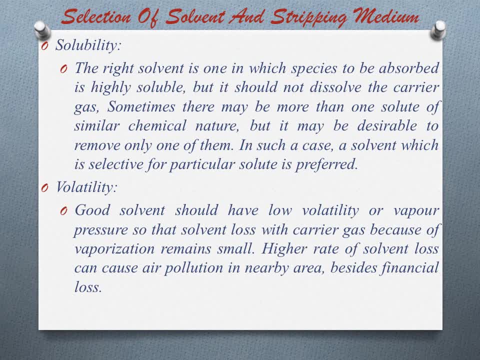 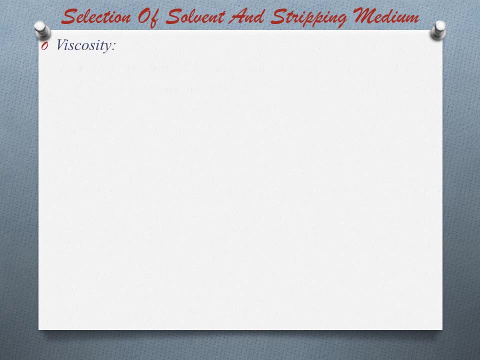 or vapour pressure, so that the solvent loss with the carrier gas because of vaporization remains stable. A higher rate of solvent loss can cause air pollution in the nearby area, besides financial loss. Then viscosity: A solvent should have a low viscosity so that it flows easily. A viscous 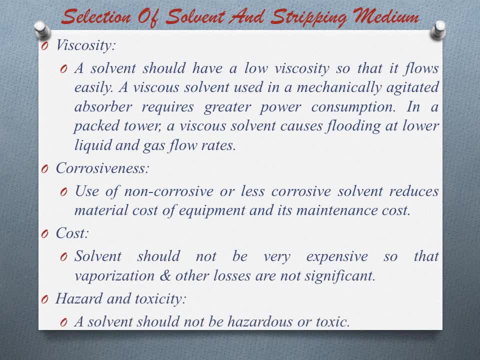 solvent used in a mechanically educated absorber requires greater power consumption. In a packed tower, a viscous solvent causes flooding at lower liquid and gas levels. Use of a non-porosive or less porosive solvent reduces the material cost of the equipment. 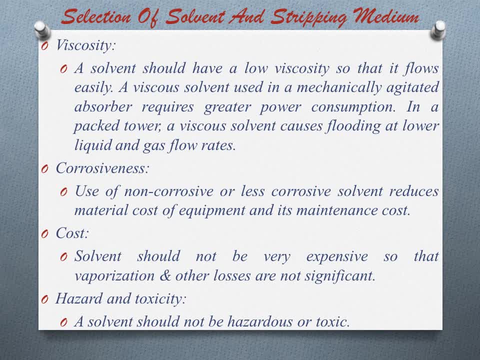 as well as its maintenance cost, Then its cost. A solvent should not be very expensive, so that vaporization and other losses are not significant in terms of economy. Next is Hazard and Toxicity. A solvent should not be hazardous or toxic. A solvent should 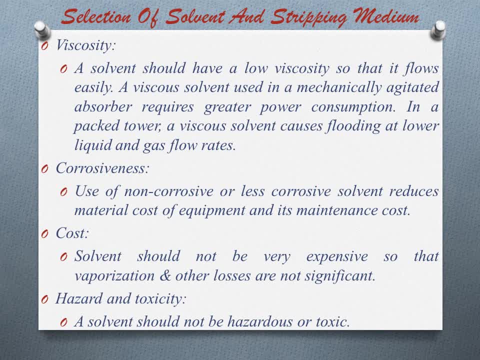 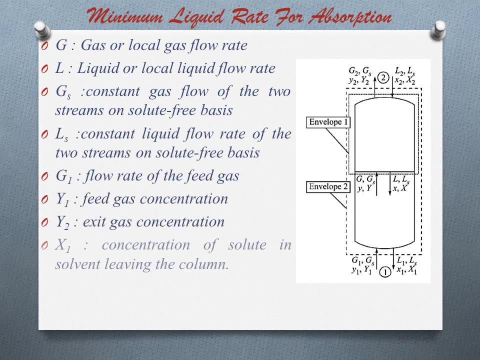 be not inflammable. Now the question is how to determine the required solvent flow rate for a given absorption problem. Let G refer to the gas and L to the liquid. These symbols also represent the local gas and liquid flow rates respectively. in the column, GF and Ls are the constant rate of. 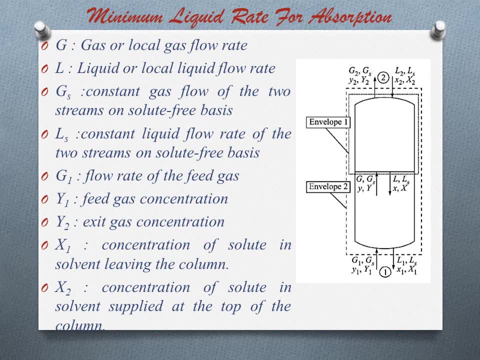 flow of the true stream to the next flame. GF is the current rate of Gs and L is the constant of the true stream on solute free basis, ie Gs and Ls are the flow rates of the carrier phases. G1 is the flow rate of the feed gas. Y1 and Y2 are the peak and exit gas concentration. 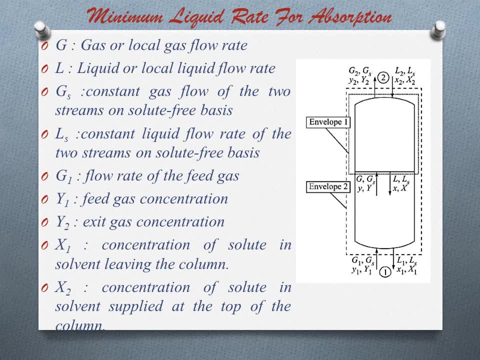 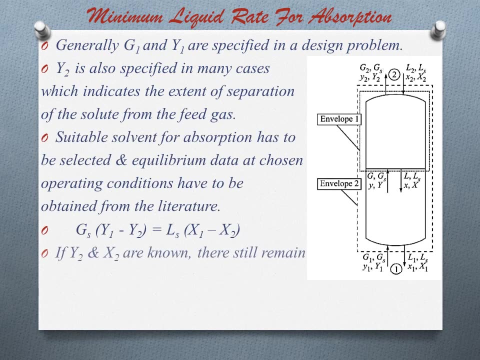 respective X1 and X2 are the concentration of the solute in solvent leaving and supplied to the column respective. In gas absorption calculation, the flow rate of the feed gas G1 and its concentration Y1 are generally specified in a design formula. 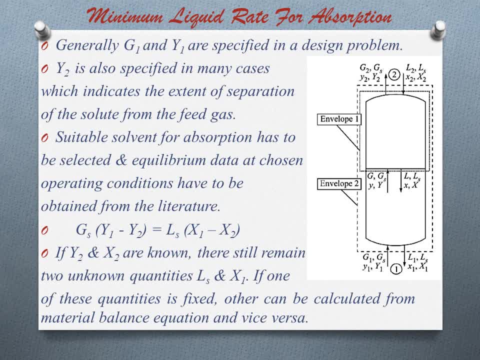 The exit gas concentration, Y2, is also specified. in many cases, Y2 indicates the extent of preparation of the solute from the feed gas. A suitable solvent for absorption has to be selected and the equilibrium data at the crucial operating conditions, ie temperature and. 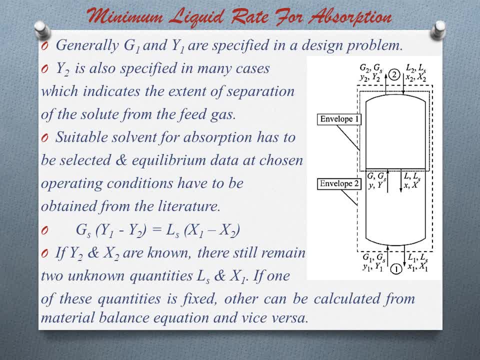 pressure have to be obtained from the literature. Now we consider the overall material balance equation ie. Gs into Y1 minus Y2 equals to Ls into X1 minus X2.. If the concentration of the solute in the exit gas Y2 and that in the solvent X2 supplied at the top of the 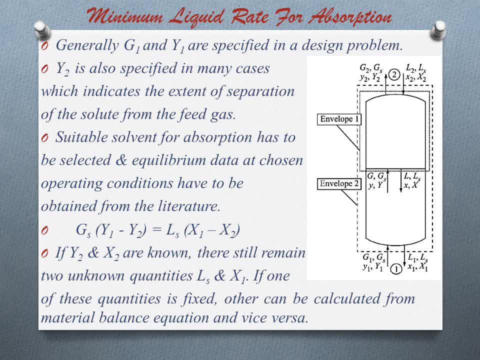 column are known, there still remains two unknown quantities: Ls and X2.. If one of these quantities, say Ls, is fixed, the other- for example X1, can be calculated from the material balance equation and vice versa. The operating line can then be drawn. 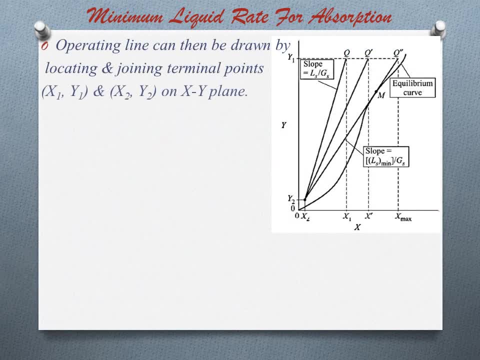 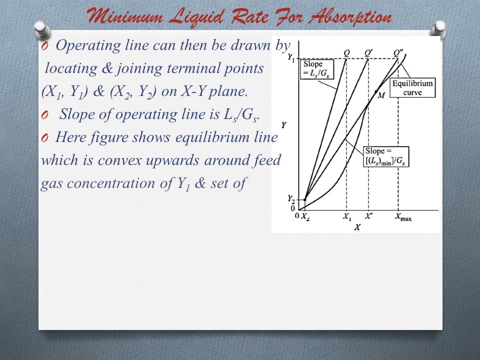 by locating and joining the terminal points X1, Y1 and X2, Y2 on the XY plane. The slope of the operating line is Ls by Gs. If Ls is reduced, ie a lower liquid concentration rate is used, the slope decreases and the operating line PQ having one fixed terminal. 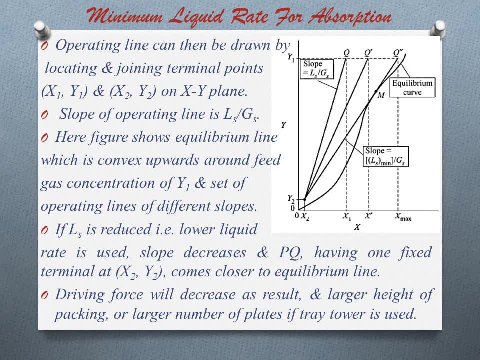 at the point X2, Y2 comes closer to the equilibrium line. The driving force will decrease as a result and a larger height of packing or a larger number of plates, if a tradeover is used, has to be provided to achieve the desired degree of separation. But we cannot keep on. 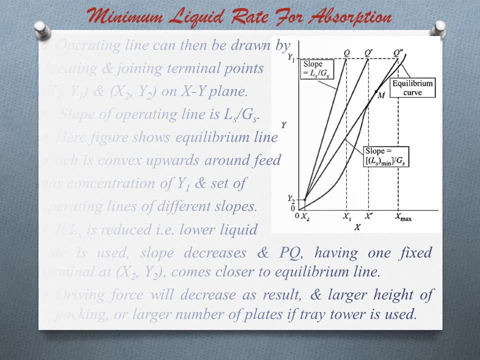 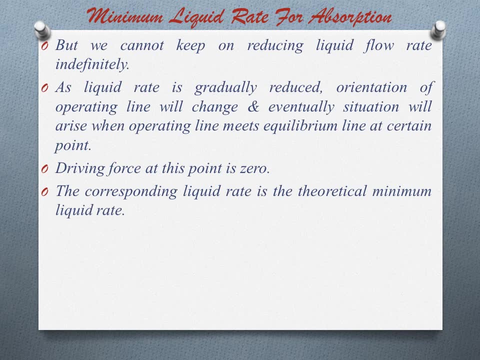 reducing the liquid flow rate indefinitely. As the liquid rate is gradually reduced, the orientation of the operating line will change and eventually a situation will arise when the operating line meets the equilibrium line at a certain point. The driving force at this point is zero. The corresponding liquid 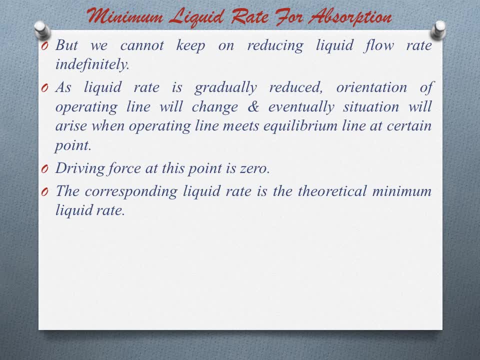 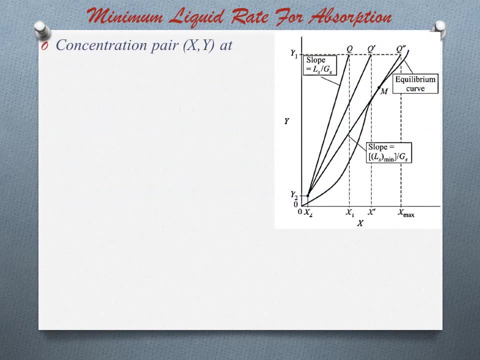 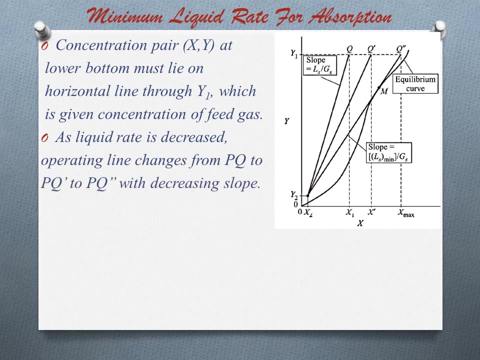 rate is a theoretical minimum liquid rate. As in figure, the equilibrium line is convex upwards around the feed gas concentration of Y1.. The concentration pair XY at the lower bottom for absorption must lie on the horizontal line from Y1, which is the given concentration. 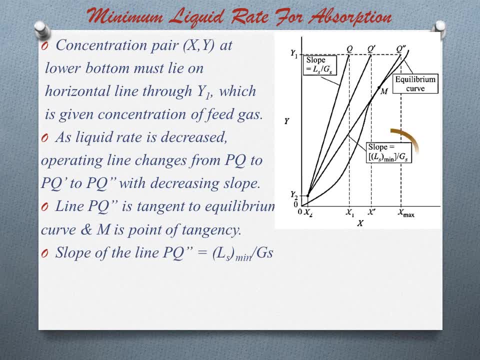 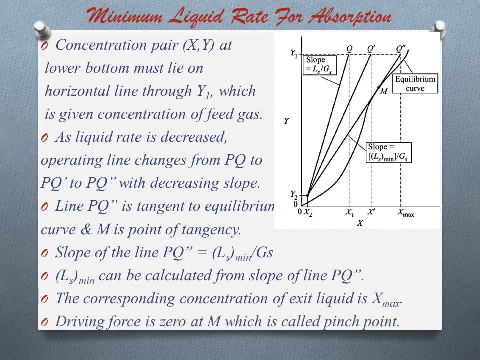 of the feed gas. As the liquid rate is decreased, the operating line changes from PQ to PQ' to PQ'', with decreasing slope. The line PQ'' is tangent to the equilibrium curve and M is the point of tendency. So slope of the line PQ'' equals to Ls minimum by Gs, Since Gs, which is the flow rate of, 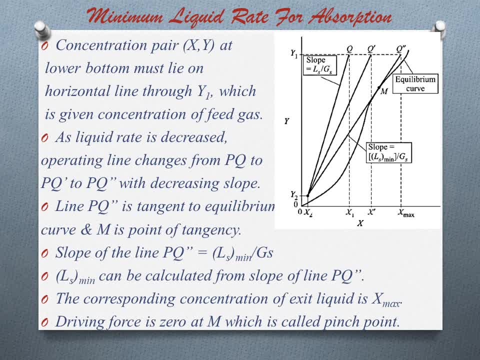 the carrier gas is low. Ls minimum can be calculated from the slope of the line PQ''. The corresponding concentration of the exact liquid is X maximum, Which is the maximum possible concentration of the liquid. The driving force is zero at the point M, That is the point of tendency for the particular shape of the equilibrium. 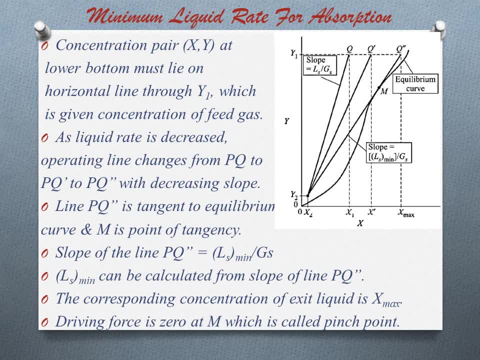 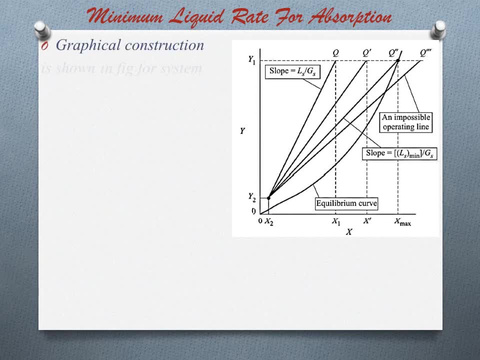 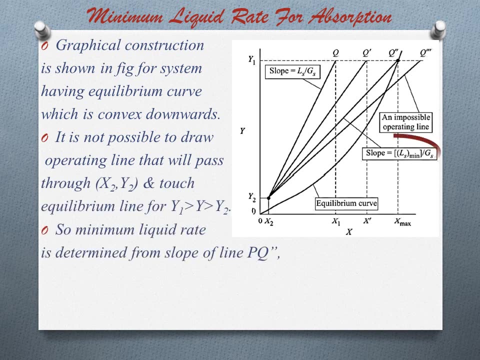 line, which is called the pinch point. The graphical concentration is shown in figure for a system having an equilibrium curve which is convex downwards. In this case it is not possible to draw an operating line on the equilibrium curve. The equilibrium curve is the slope of the point Q'' that will pass through X2 and touch. 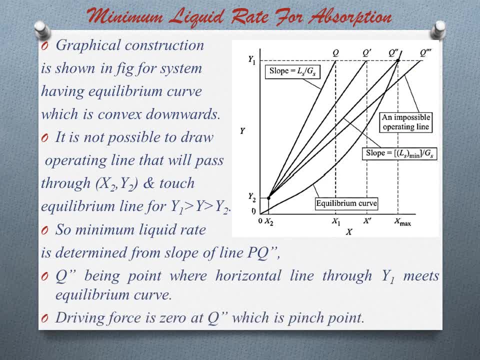 the equilibrium line for Y1- Y2.. So the minimum liquid rate is determined from the slope of the line PQ'', where, Q'' being the point where the horizontal line through Y1 meets the equilibrium curve, The driving force is zero at the point Q'', which is the pinch point. 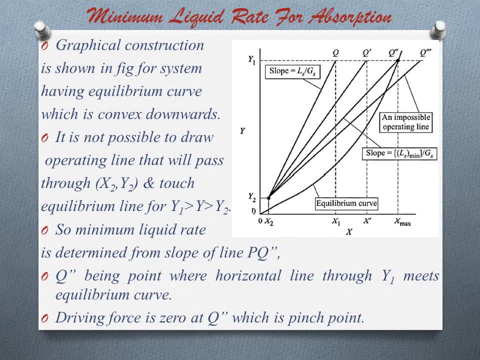 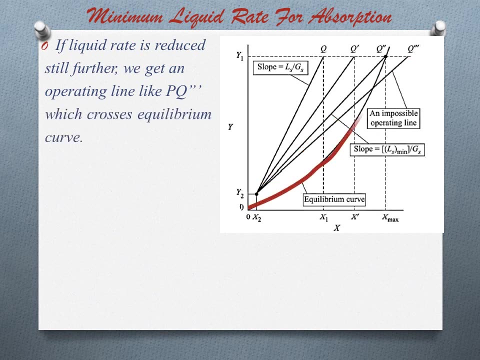 in the equilibrium curve, which is the pinch point in this case. If the liquid rate is reduced still further, we get an operating line like PQ triple dash which crosses the equilibrium curve. This is physically impossible. A line like PQ triple dash cannot be an operating line. So PQ triple. 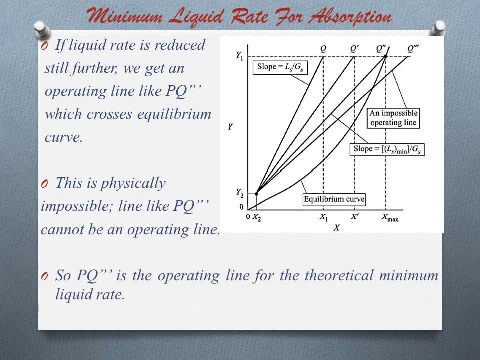 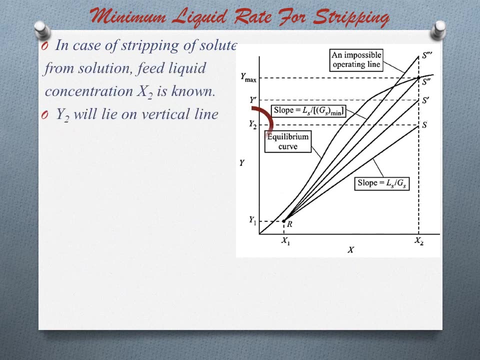 dash is the operating line for the theoretical minimum liquid rate. In the case of stripping gas of a solute from a solution, the feed liquid concentration, X2, is low, So Y2 will lie on the vertical line, so X2.. The lean liquid leaves the column at a concentration of X1. 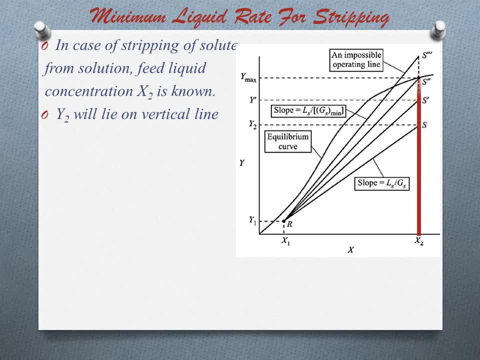 and the stripping gas concentration is Y1.. The points are: that is X1 to Y1 represents the bottom of the tower. If the stripping gas is free from the solute, it is Y1 equals to 0. So let GS be the flow rate of the stripping gas on solute-free basis. If we keep on reducing, 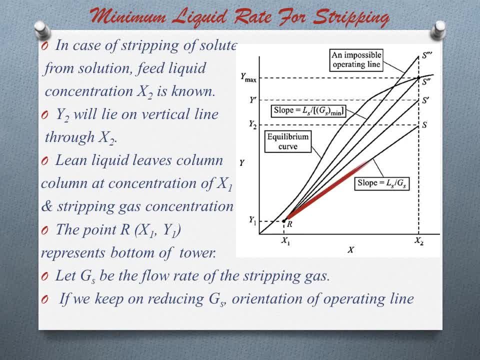 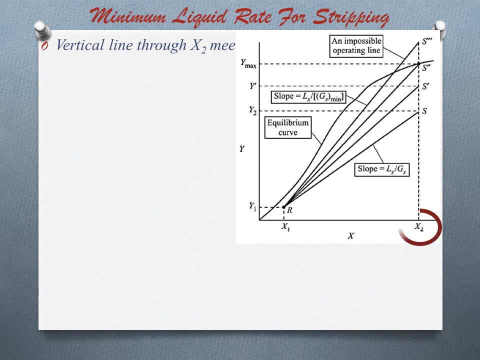 GS. the orientation of the operating line changes from RS to RS single dash to RS double dash with a gradually increasing stroke. The vertical line through X2 meets the equilibrium curve at S double dash and RS double dash, which is the opposite. The operating line for the minimum stripping gas rate, GS minimum, The corresponding solute. 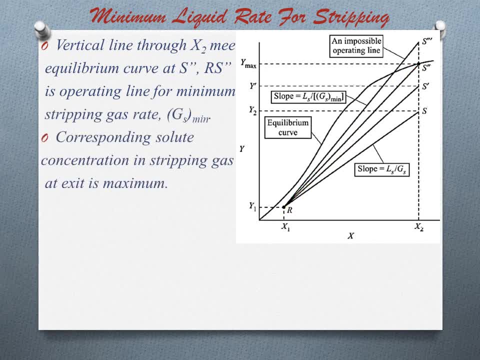 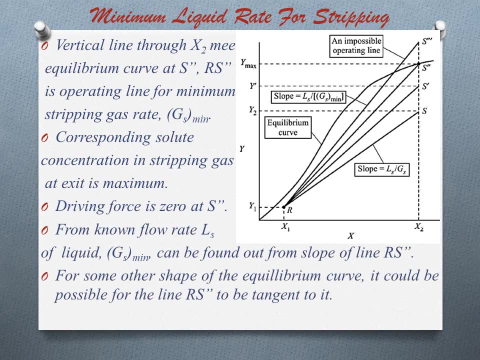 concentration in the stripping gas at the exit. gas is the maximum via maximum. The driving force is 0 at S double dash. It is the pinch point From the known flow rate, Ls, of the liquid. the minimum gas rate, GS minimum, can be found out from the slope of the line at the exit. 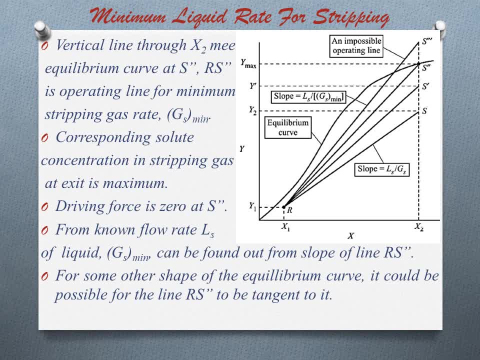 gas. For some other shape of the equilibrium curve, it could be possible for the line RS double dash to be tangent to it. In such a case the point of tendency would be the pinch point. It all depends upon the shape of the equilibrium curve. A line like RS triple dash 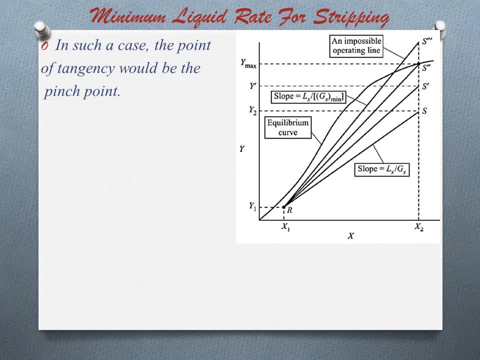 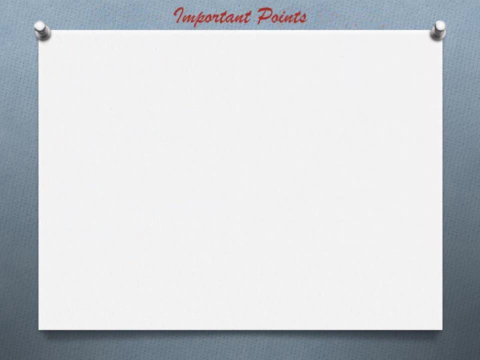 in figure crosses the equilibrium line and cannot be an operating line. The line can not be an operating line. A few more points have to be noted. In any practical problem, the pinch point does not occur at the top end of the column for absorption or at the 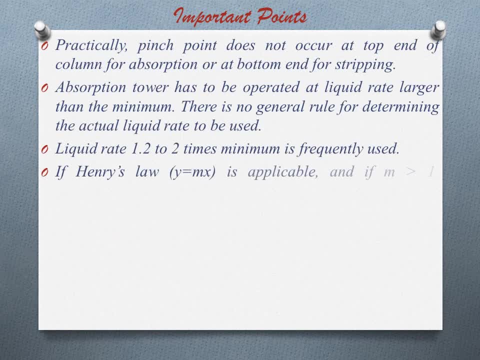 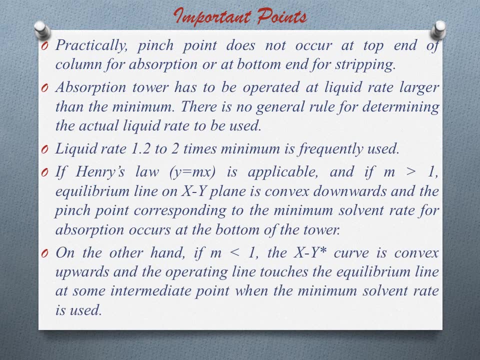 bottom end for stripping An absorption tower has to be operated at a liquid rate larger than the minimum. There is no general rule for determining the actual liquid rate to be used. However, a liquid rate 1.2 is the minimum liquid rate. The minimum liquid rate.